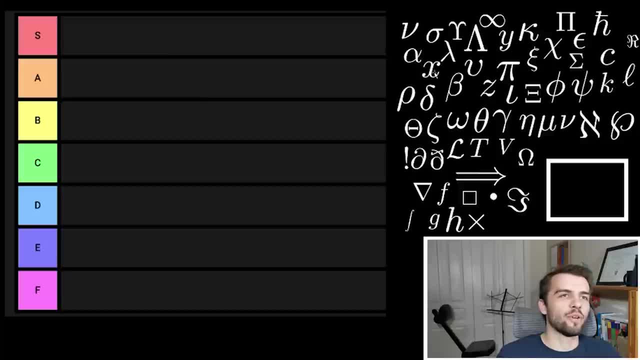 suck. Some of them are really good. Let's get started. Alright, first up is the classic. You got X here. Imagine if you were told: alright, you can do math, but you can never use X again. right, You'd probably be pretty broken hearted about that. So X, you know, it's nothing like. 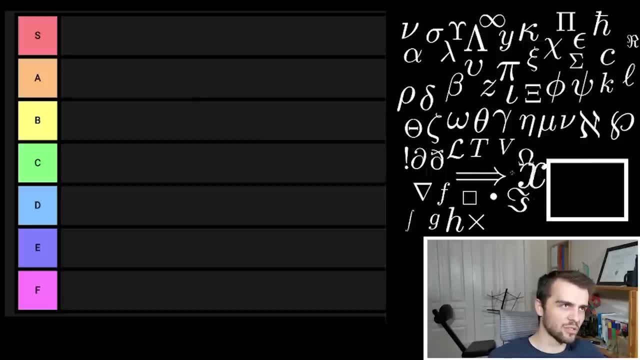 super special. It's not the best symbol ever, but it's essential, So I'm going to put it in A tier right here. Along with X, of course, comes Y. These are like the basic, basic symbols of math. You really can't do anything without X and Y. And if I was told, I couldn't use X and Y again. 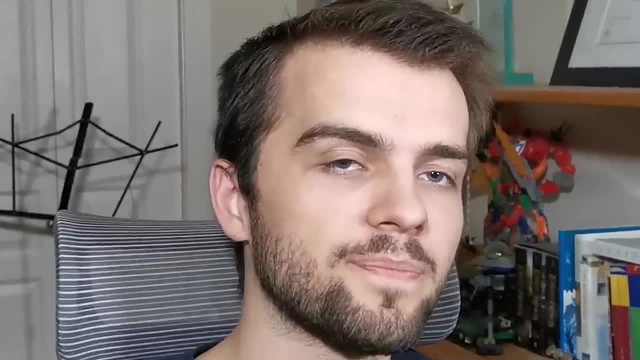 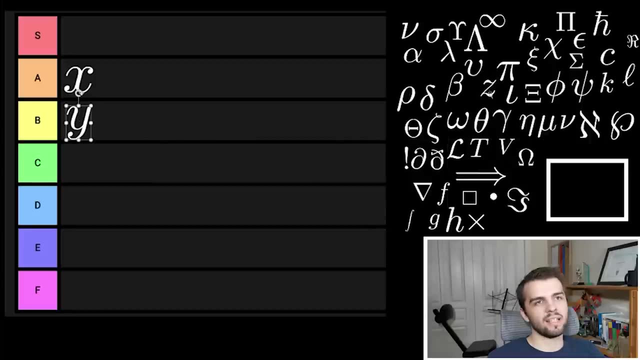 I honestly don't know what I would do. I would drop out. I would join biology. So Y pretty good, Not quite X. right, You don't use Y in quite the same situations. Y is going to be B tier And like Y, of course, you have Z here, Z being the third Cartesian coordinate, A nice. 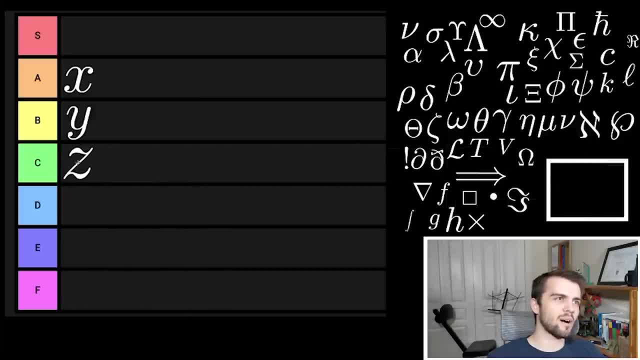 looking symbol. right, These are all nice, nice looking, But I'm still going to put it probably in the C tier here. Now here's a beauty here. We got Alpha And I like Alpha. You know it's kind of hard to write when you first start learning to write it, But it could be maybe I just like Alpha. 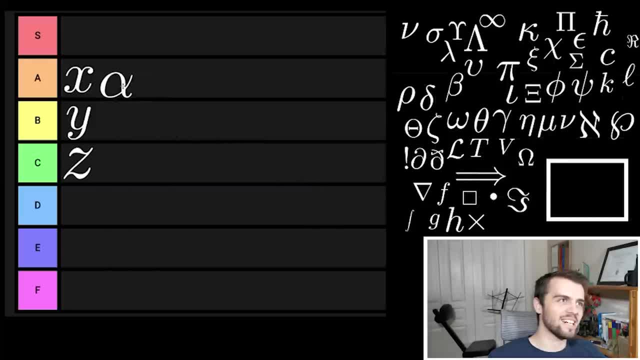 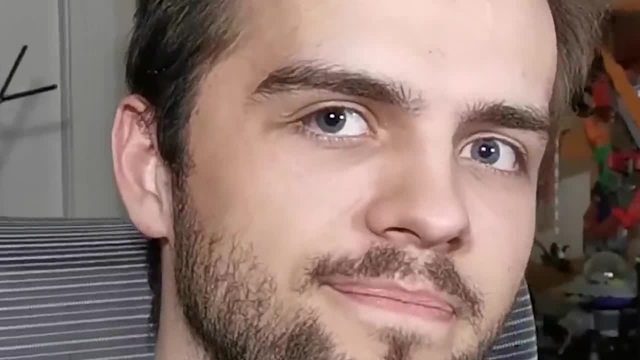 because I am one Alpha. I'm going to put that in the A- B tier right here. Beta, of course, is the next letter in the Greek alphabet. Of course I don't like Beta because I'm not one. Beta shows up like Alpha when you're writing the angle of things: a. 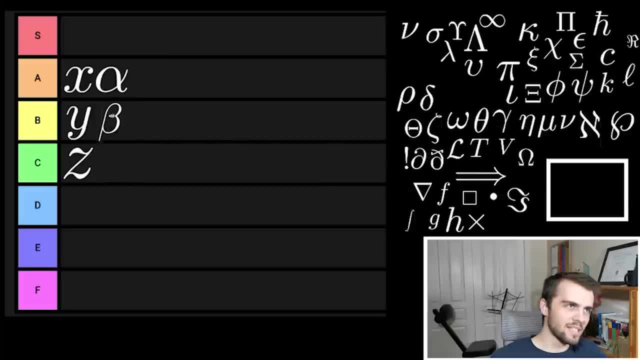 lot. So you know I'm going to put Beta in the B tier And there's a pattern here. but no, don't, don't even think that I'm just going to choose random Here. we got capital Pi. Capital Pi is. 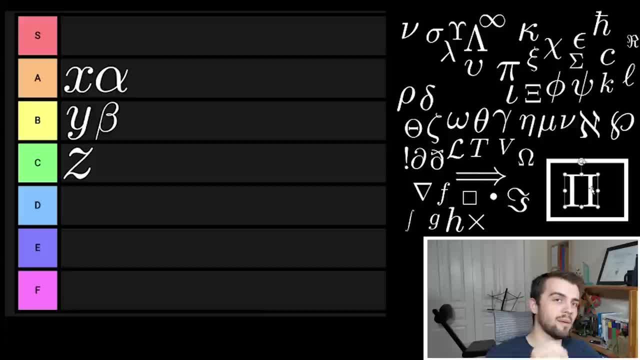 like: pretty cool, I didn't even know it existed for a long time. Maybe you didn't know it existed either, But it's like the product of a bunch of things. So if you're going to write something, if you have a bunch of, you know, variables or whatever, you take capital Pi, take the product. 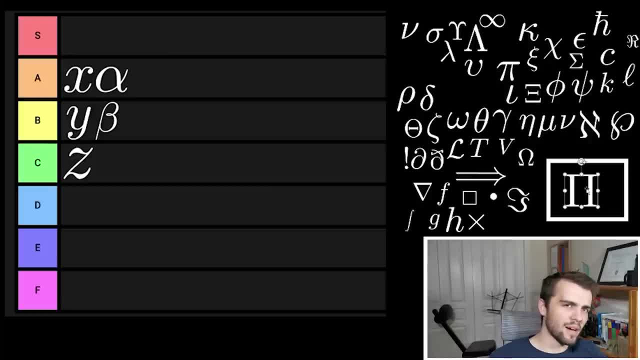 of them. Pretty cool stuff. You know you can do that. That's allowed in math. I'm going to put Pi as an A tier because of its computational functionality. Next we got infinity, And now infinity is pretty big. There's lots of infinities. There's the infinite love I have for physics, Just 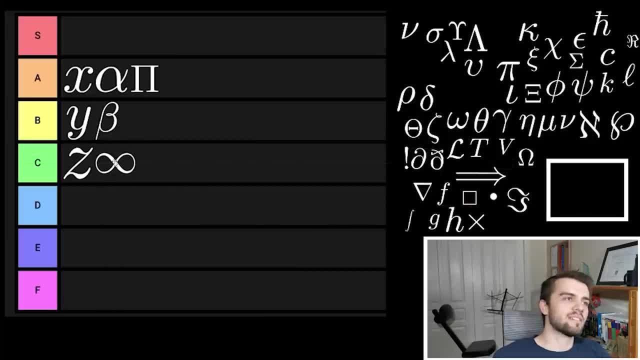 kidding, That's definitely finite Infinity. I'm going to put it in as a C tier. It's kind of just like an eight Rotated 90 degrees. So whoever came up with this, you know, got to be more creative than that. Two: 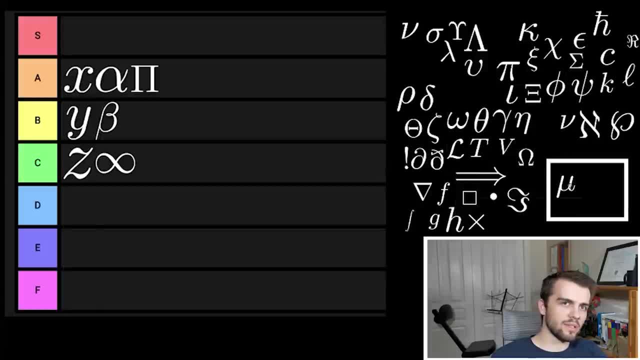 symbols. I hate Not this symbol, these symbols mu and u. And now mu and u can actually go die in hell together, because whenever they're used together on the same thing, you always mix them up right, They're the same thing. Who is it? who's coming up with all these shapes that have you? 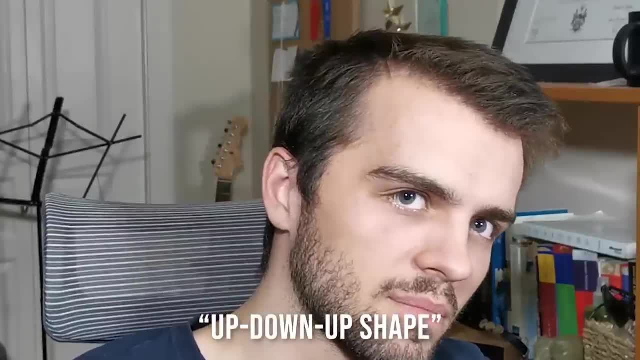 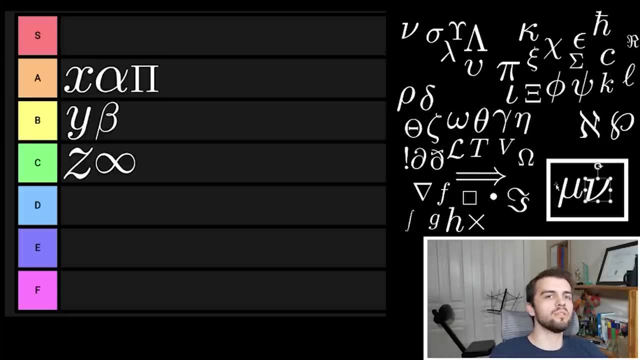 know this. you know up down, up shape to them. Both of them are like that. You got to be more creative and don't use them together. And I always hate, for some reason, whenever someone wants to use mu, they're also using mu. Yeah, They look. 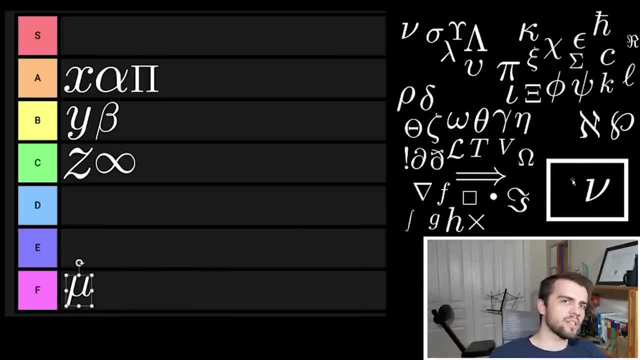 different here. Try writing them down and you'll confuse them. So both of these are F tier for lack of creativity. Mu is just a U with a thing here. All right, next up, chi. Now, not to be mistaken with X, chi is a pretty cool symbol because chi always represents something like cool, like the. 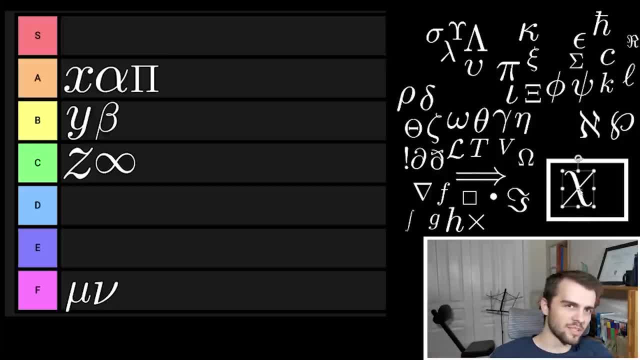 chi squared distribution. So I associate it with like good things in my mind. i also like it how this is like really thin and then this line is thicker. it gives like kind of a dimensionality to this symbol. uh, i'm gonna put kai is a tier for. 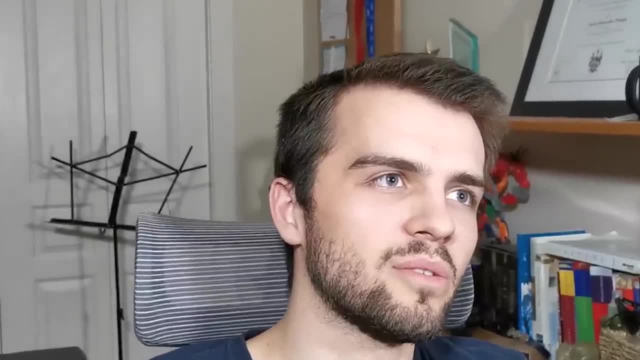 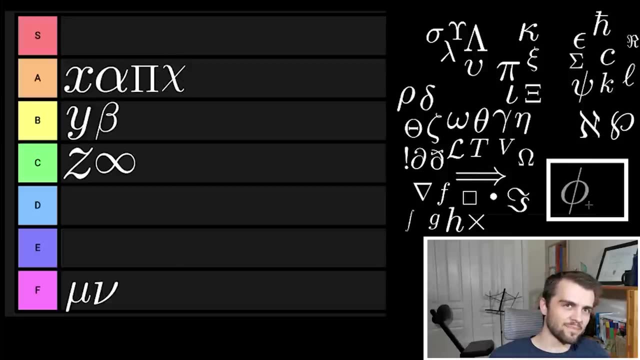 being just like you know. you're a cool dude, you, you represent cool things and i like you and you're welcome in the a tier. all right, phi, phi is classic. phi is like um, i think theta is like x and phi is like y. for angles it's like okay, theta is not being used, so you got phi and in that sense, i. 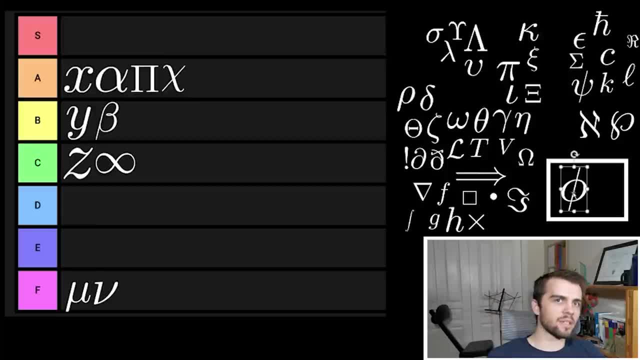 think phi is b tier simply because theta is probably going to be a tier. in fact, i'll put theta wherever it is a tier, because that's like the go-to angle. right, that's your guy and you're like, oh, theta's taken up. well, i gotta go to my, you know, second in command, or whatever, phi. all right, 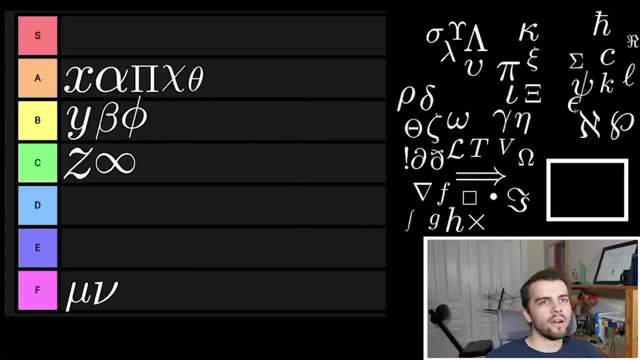 i gotta use phi. now i've got more symbols. phi b tier, all right, epsilon. epsilon is an interesting symbol. epsilon always shows up in things where you're annoyed, if like, oh, now you're dealing with something small, so now we're gonna put an epsilon. think epsilon is something small, now we're gonna do a math proof. that sucks, i'm. 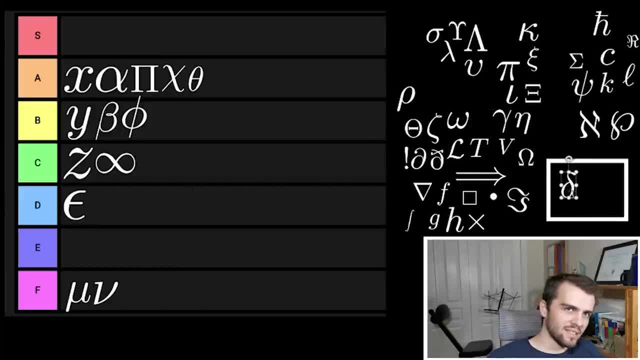 gonna have to put it in d tier. all right, delta. now delta is kind of similar. delta also shows up when you're confused and equations are bad, and then they're like: okay, now delta, and we're gonna do something weird that you've never seen before, and delta is somehow going to be responsible for it. 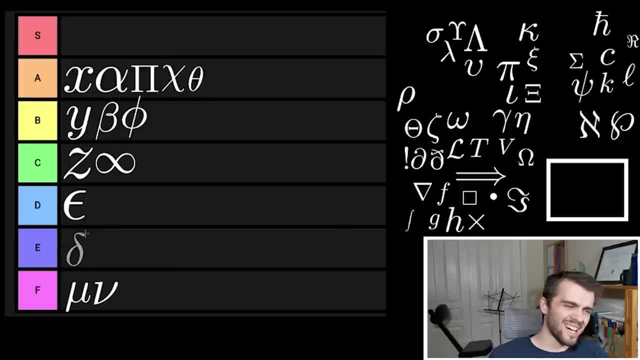 e tier. it's kind of a cool symbol, but it just shows up at the wrong time and i'm sorry, dude, you show up at the wrong times. you get put in the e category. that's how it works. sigma's kind of like just bland. i don't know what it is, but there's something really bland about this. 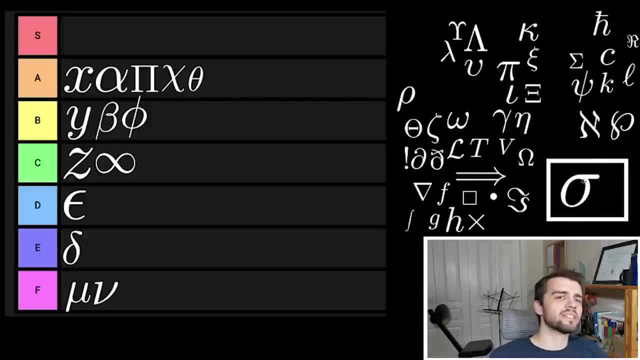 symbol. i don't see anything really fascinating about this symbol. in fact, it shows up sometimes and i always think, well, couldn't use a better symbol. i'm gonna put it in d tier for sigma, all right, i've never seen this symbol before. i'm gonna call it the coat hanger symbol. 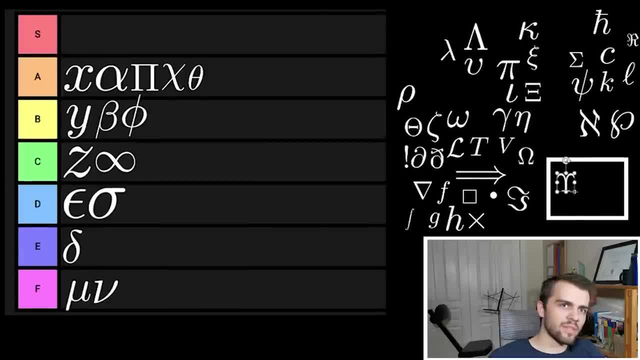 um, i don't particularly know if it's ever been used ever and anything in math. it somehow is in latex and i grabbed it and here it is and i don't know who you are. you're like a mystery man and i think it would be cool if people used you sometimes. 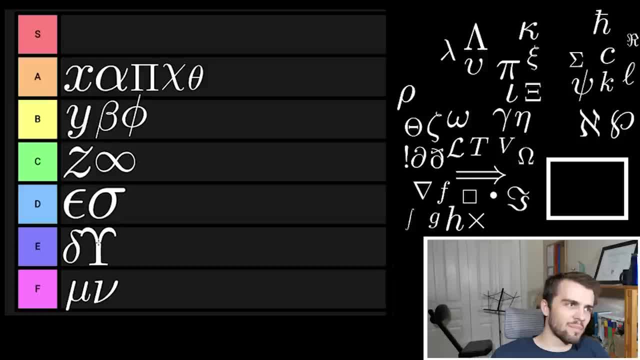 for being like mysterious. um, you know i'm gonna have to put you in e tier, but just because you've never been used before, you know you don't belong in a very good tier. all right, kappa kappa's kind of cool. it's like a k. it's kind of bent, like it looks like it's out of shape or something like. 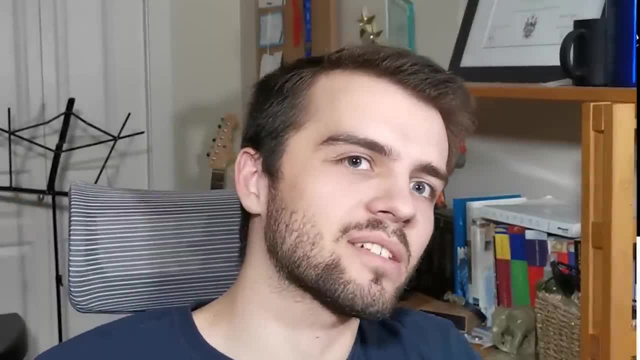 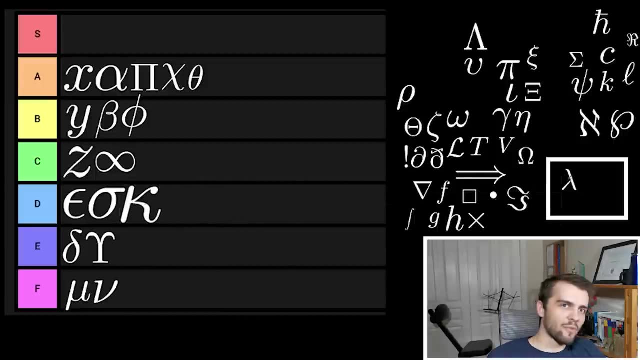 something happened to a k. it got whacked with a stick and now it's all bent and kappa's definitely a d tier. it's not great, but it's not fantastic. i feel like lambda is kind of one of the first symbols that you ever deal with, where 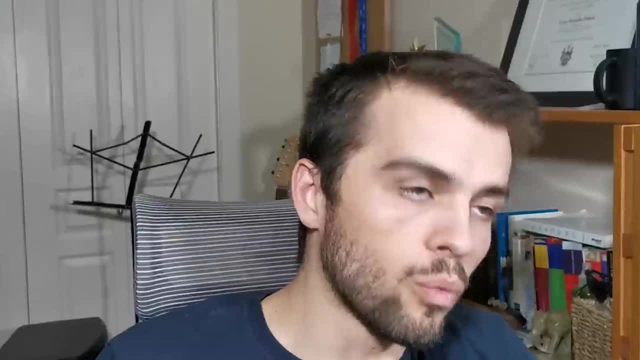 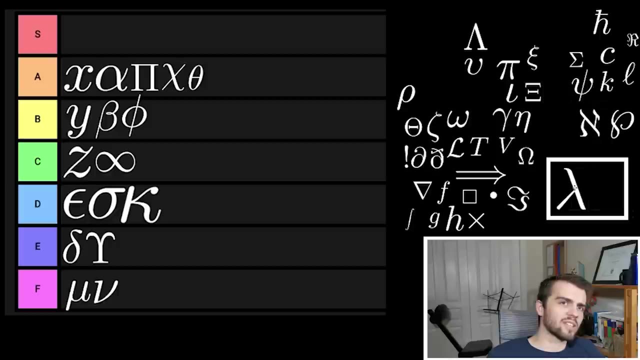 you're kind of like beyond x and y and you're in physics and it's like: oh, we're going to talk about wavelength, we're going to use this new symbol and you get all panicky because you've only used three symbols before. all of a sudden you're using lambda. it doesn't even look like. 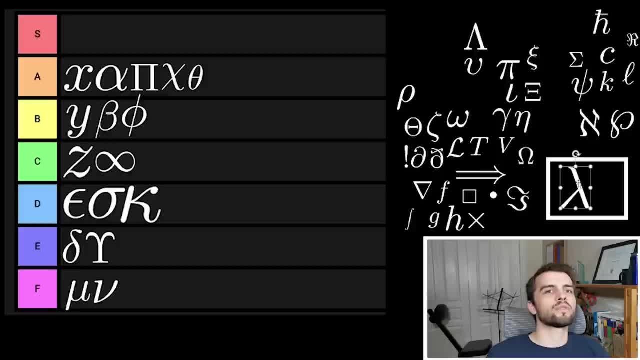 anything you've seen before. but i have to give it points for being like structurally um integral right. i mean it's living in two dimensions, it's leaning, it's got this extra support here so it doesn't fall over. i'm gonna put lambda b tier. it's nothing great to look at, but 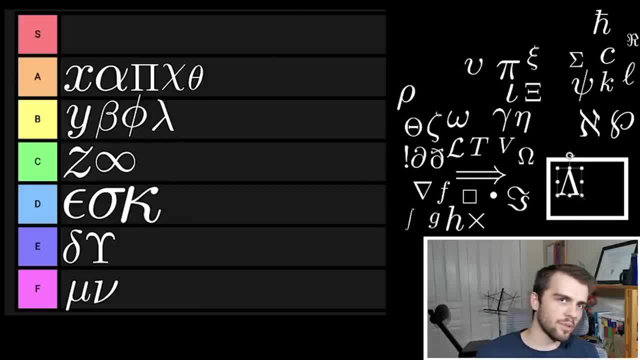 it's. it is what it is: capital lambda. capital lambda. now, i think this is the most underrated symbol ever. you have all these symbols and all this fancy crap that you see all over the place, and even in the english alphabet, and they didn't think to make this a symbol. 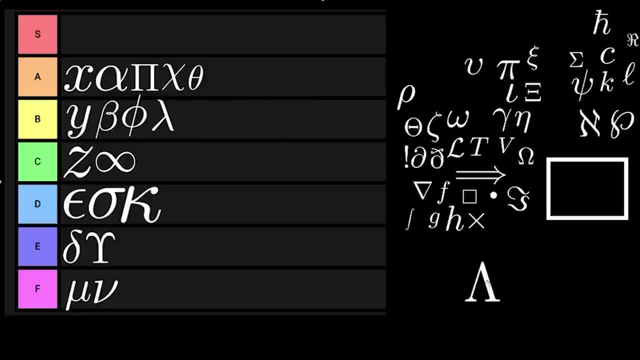 it's even simpler than an, a, a capital a, and it's not used. everyone wants to do their u's and v's, mu and nu and all this crap in the f tier. no one thought to do it the other way and it's so simple, right? why not make the first letter of the alphabet this thing here, this capital lambda? 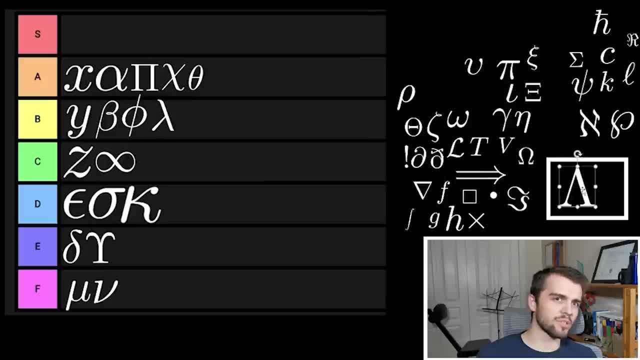 what a beautiful underrated symbol. and for being so underappreciated, i'm going to put you in the a tier. you're, you're cool and you should have been here. okay, and you're not used as often as you are cool looking symbol, especially in latex. it's got that like horseshoe vibe. it's got kind of a. 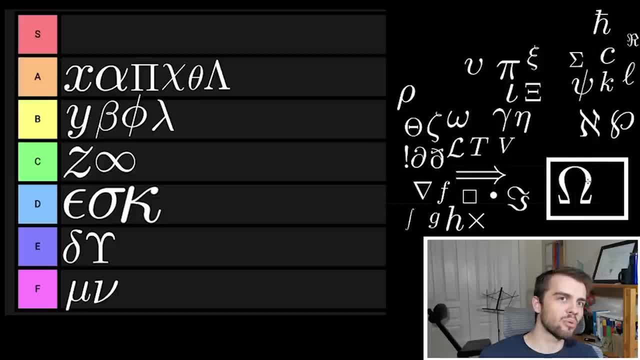 like you know, mysterious support arch vibe. i'm gonna put it beet here, but probably be tiered just because it's not used very often. i wouldn't even use it really. here we got another one of these mu nu nu symbols. it's it's even different than those. 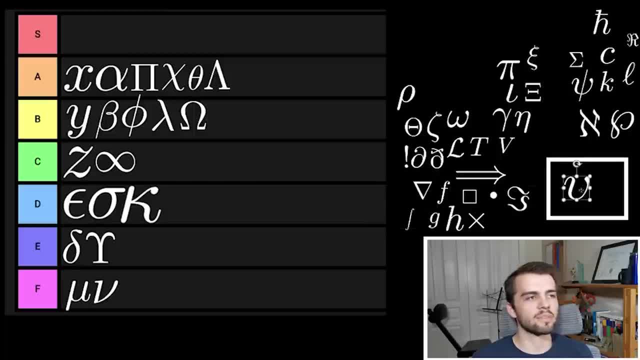 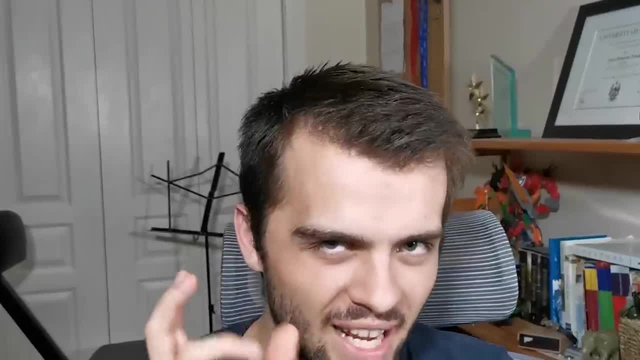 two. i don't even know what this is called here. probably another one of this crap, so It belongs here with these. Look, they're all basically the same. Could you imagine using all three of these symbols at the same time? It's not that any one of them is bad. 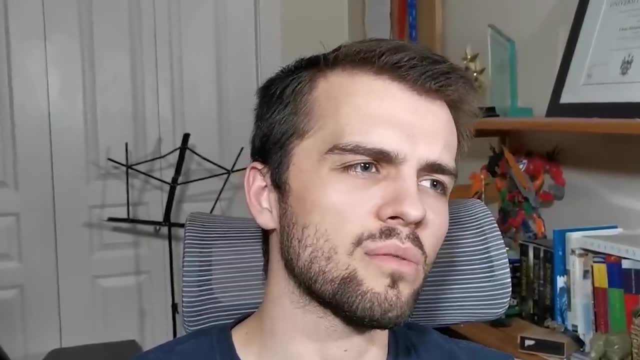 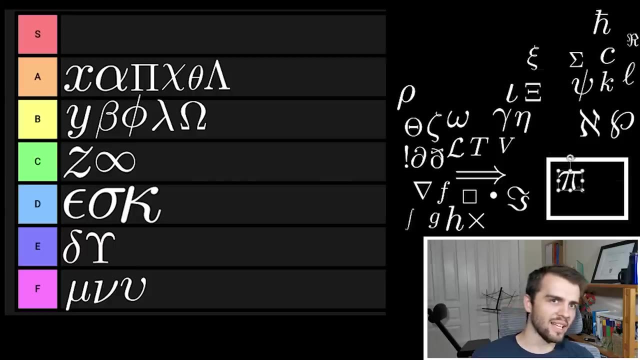 but it's just they get mistaken all the time. Don't do this. Don't have three things that look like this Math. why are you this way? The symbol pi: I like the symbol pi. It's kind of an important number. 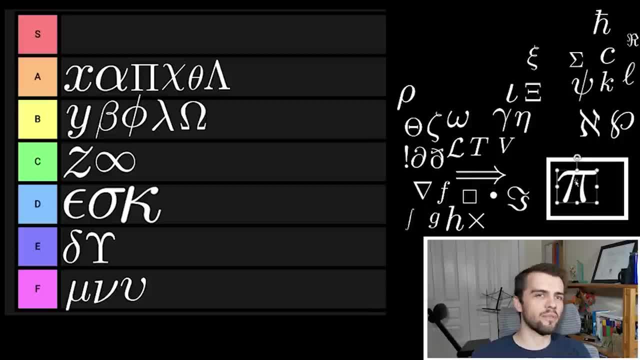 I don't know if you've heard of it before, And it's so important for everything that I think it's gonna have to go in S tier. I mean the history behind this number and calculating it, and it shows up all the time. 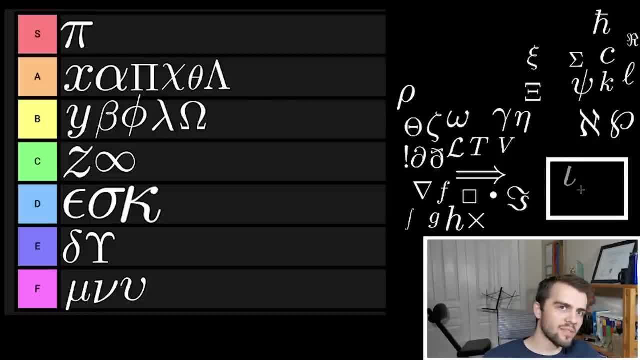 that's really an S tier number. I don't know what this is. I've never seen this before. I'm glad it's not used. It's just overall awful. I think this again belongs in F tier. I think it's iota or something, but it's just no. 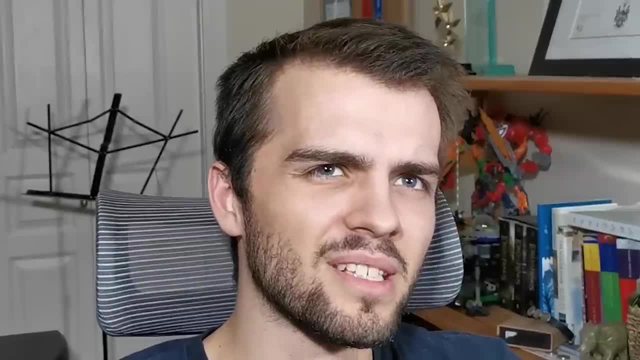 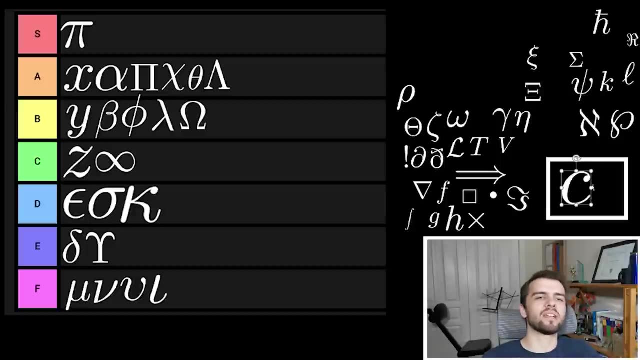 It's got the same sort of shape, this U shape. Just stop with these C. C is like representing the speed of light in physics. C is so important. The history behind this symbol and everything too, but honestly, C tier. 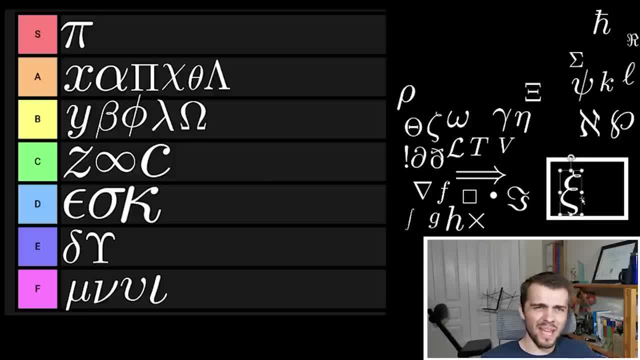 This symbol here. I've seen it used in papers. People love to use it because it's like: look at me, I'm a fancy guy. I use fancy symbols that have curls like this and have no purpose. I could have used something else. that's way simpler. 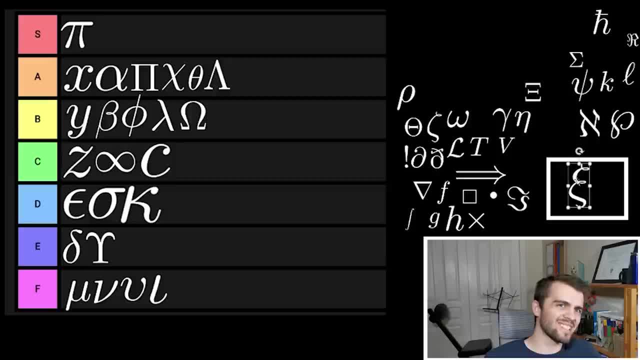 but I use this fancy curly symbol that also takes up a lot of space. It's so pretentious and it's overused, and it's like wearing a purple hat with a feather in it. It's just No, it's too fancy, not for me. the E tier right. 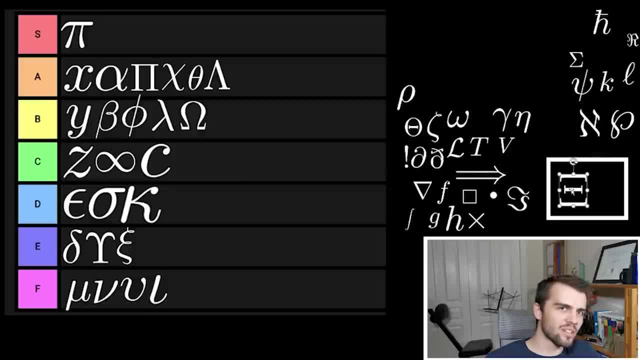 This is another one of these things I've never seen used and I'm really happy it's not used, because what a pain to write. To take your hand up three times and write three things in for one thing is too much. This is an E tier item. 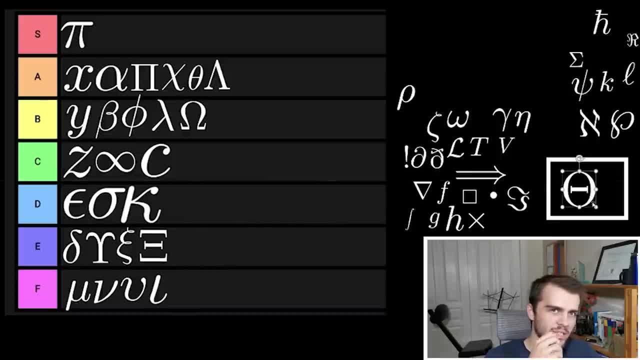 All right, here we got capital theta and capital theta is again one of these things I've only seen come up recently and it's different than theta, and I kind of hate it because I used to have trouble differentiating it between theta and theta. 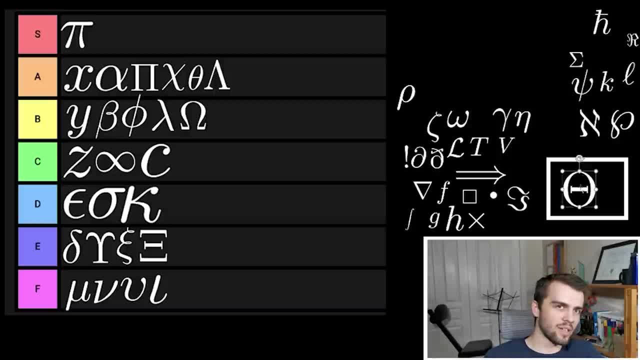 but what I do is I lift my hand above the paper to draw this thing in the middle. but it's kind of a pain of a thing. I think it's a D tier because it's not really used that often, and if you do use it it's sort of annoying. 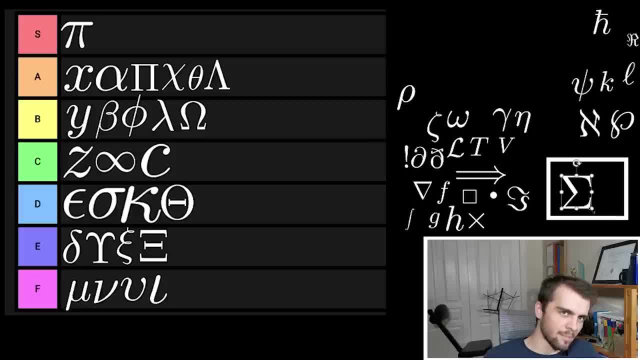 Sigma's a pretty cool symbol. Just because it's unique, it's sharp, it gets to the point. It almost looks like it would hurt to touch it because it's kind of got claws to it. I think sigma's an A tier. 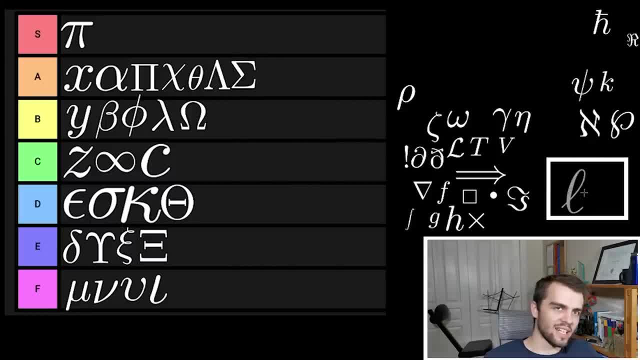 Now I actually love little L. This is slash L and it's different than L and it's just beautiful. L shows up all the time in quantum mechanics for angular momentum or whatever the heck it needs to be, and it's nice having this as opposed to just a regular L. 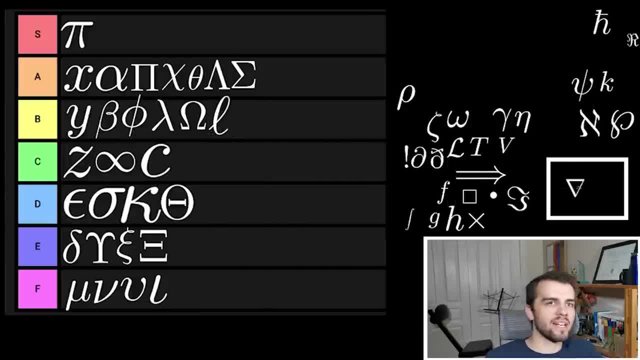 This is a good symbol. I'm gonna put it B tier, All right. next we got nabla. Nabla is an operator, It's the gradient. It can be used to represent many things If you put a little vector over it. 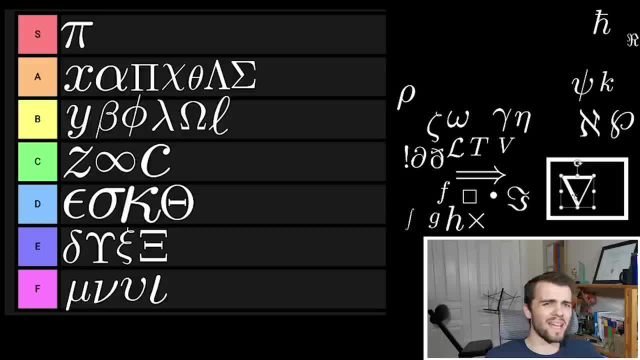 it's also a different symbol. in math It's just an upside-down triangle, very basic, but not much. There's not much to it and I kind of like that and I think I'm gonna have to put it A tier. 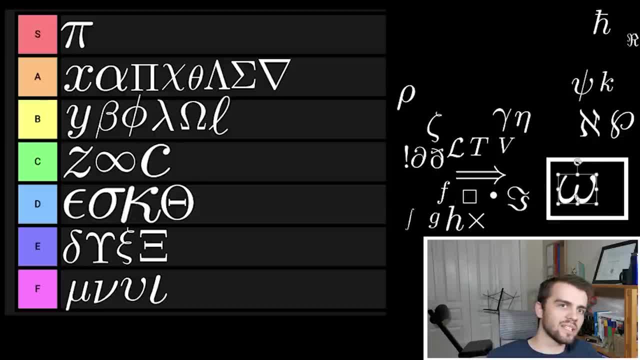 Next we got the symbol omega. Again, it looks like the W. It's kind of easy to write. It shows up quite a bit. It's nothing really special, though It's not the nicest symbol, but it does the job well. 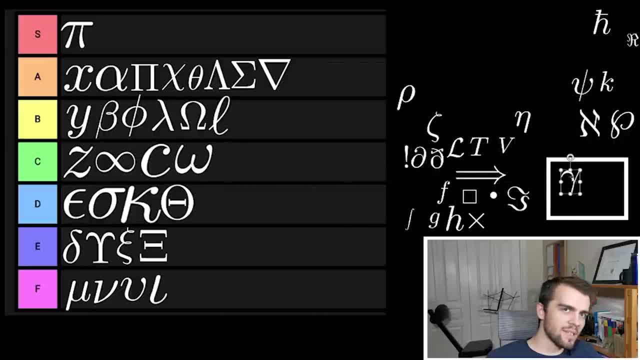 and I think omega belongs in the C tier Gamma. Gamma's an interesting symbol and I don't like the way it shows up in LaTeX here- Not the nicest. I like the little loop in it. I'm a huge fan of this particular gamma. 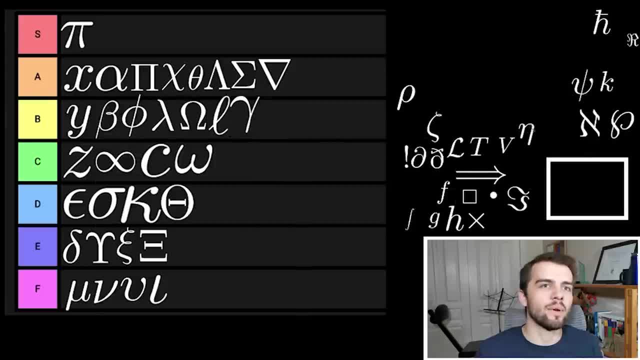 I think this is about a B tier symbol. Now we got eta and eta's kind of like mu, but it's not this F tier stuff where it gets confused a lot. I think when people use eta it's generally known what it means. 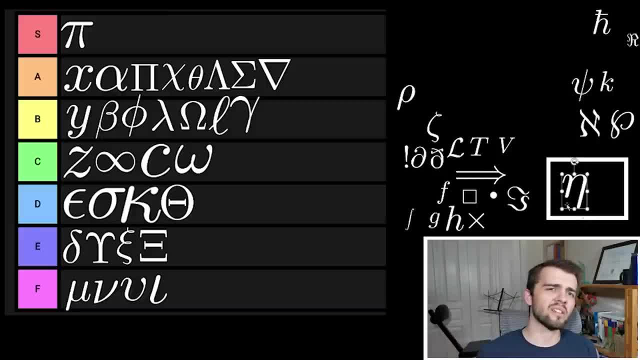 It's kind of one of those symbols that you think why not use another symbol, Why not use a little N or whatever? I don't know. I think this is a C tier, because it still has its purpose. Now we got F. 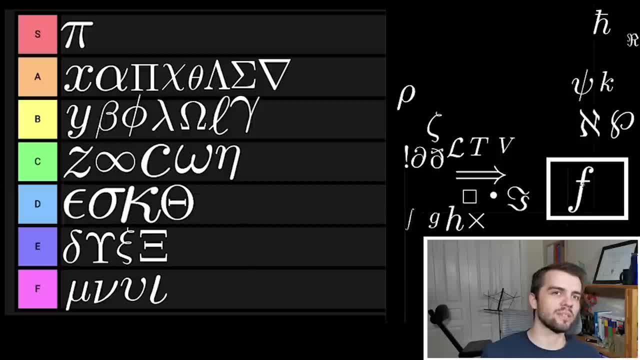 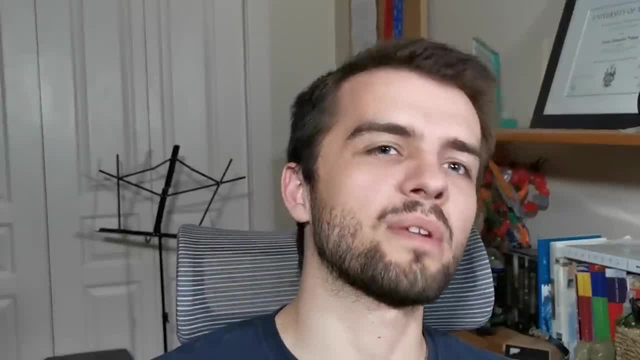 F for functions. F is a classic and I really think that there's no doubt that this is anything but the A tier, Just because of its simplicity. you have a function, You have the concept of a function, Everything is an F. 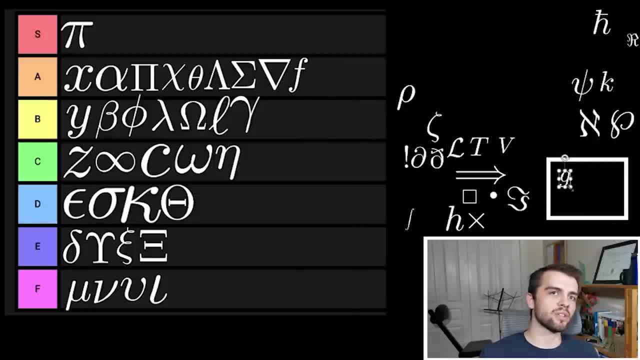 F is good. If you don't have F or if you're already using F, then you go to G. So G is kind of like the next in line to F and it's definitely not as good. It's like: oh, I guess F's used. 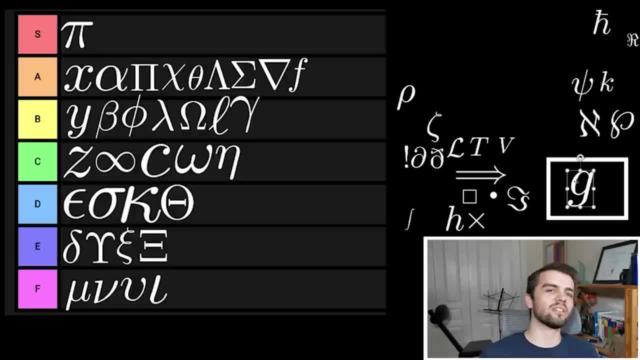 Well, now I got to use G. G is kind of lower down because you kind of look down to G. I think G is a C tier And of course, sometimes, when you don't even have G right, F and G are used. 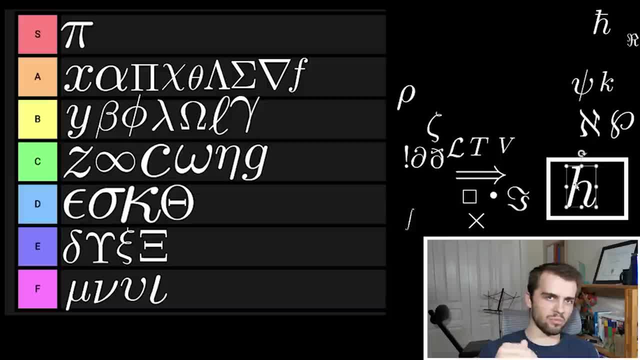 Oh, now I got to use H, And so H is kind of like below G. in that regard the hierarchy of symbols, I got to put H in the D tier. Next we have this symbol And now- don't mistake this- with an X. 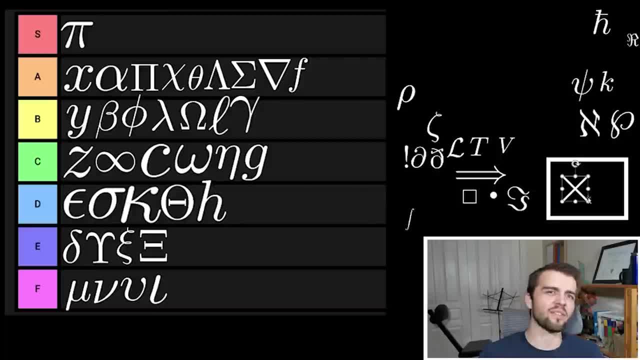 This is the cross product. It's not even times. Don't even think of it as multiplying two numbers. This is the cross product symbol. Pretty neat, The cross product, of course, being non-commutative, I'm going to have to put this in a C tier. 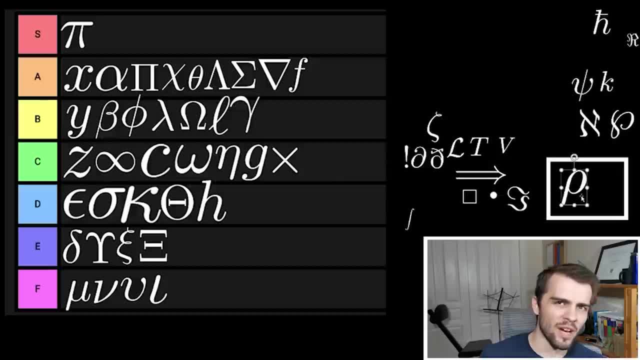 Rho is another good one. You know it's kind of dumb if you have Rho and P, They can get confused. For that I would probably put Rho C tier. I actually got this thing here. I don't know what this is. 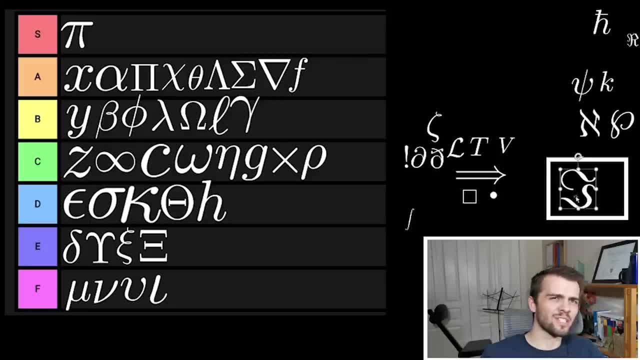 This is just like two snakes fighting or something. I think this is supposed to represent imaginary number in. for whatever reason, This doesn't read to me as anything. This is probably an E tier. Oh, we got the dot product. Ooh, the dot product is beautiful. 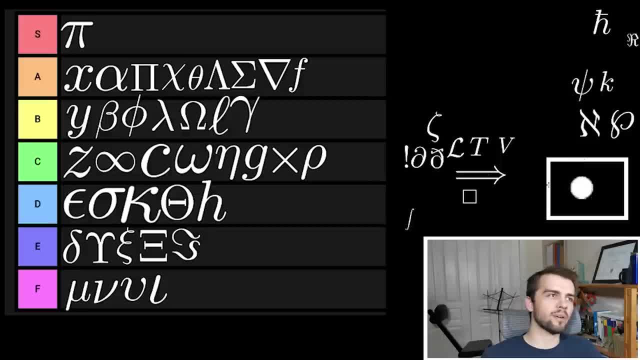 Just a nice dot. I'm going to put the dot product as B tier. It's easy to compute, It's nice, It's just a dot. Next, we got this box. I'm going to have to put this box and this box. 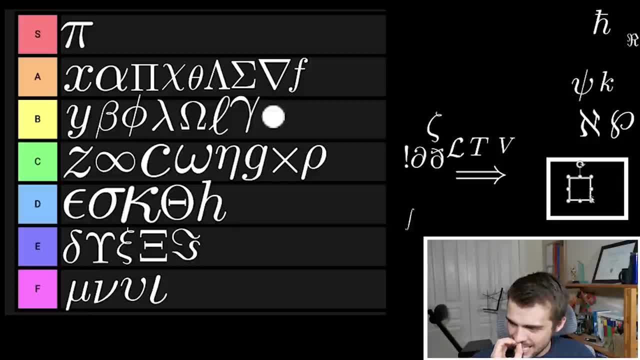 Don't be mistaken by the two boxes. This is the some symbol that represents spatial and temporal derivatives. So someone was like: I want to do this long thing that requires a lot of space. I'm just going to replace it with a box. 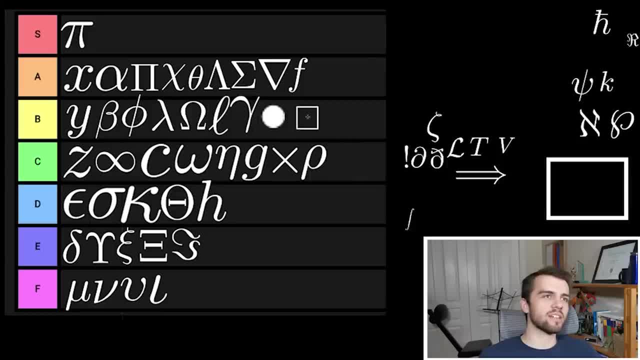 And you know what I like that ingenuity. This box here has its place in the B tier. Now, H bar is one of the classic, important symbols in physics. What a beautiful symbol. I mean, it's nothing like H, which belongs in the D tier. 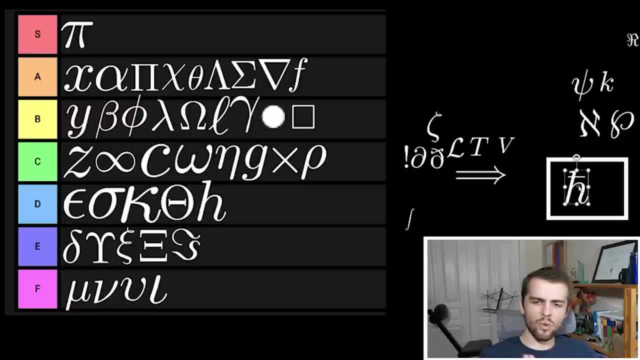 Someone said: you know what I want to represent: this number. There's no other symbol I'm going to use. I'm going to put an H, I'm going to put a bar on. it Belongs in the S tier, clearly, for its ingenuity. 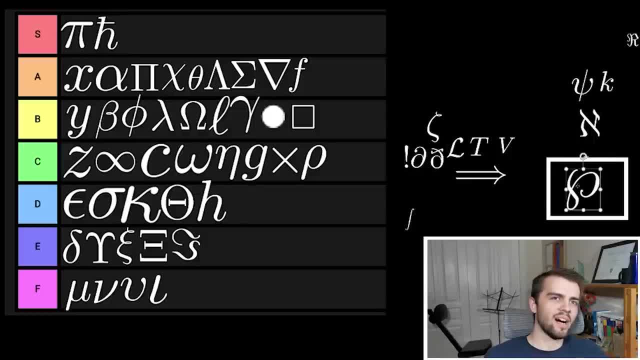 Next, we got this squiggle Again. I don't know what this is. This is just something. Again one of these. this is like this D tier. I mean, whoever came up with this probably came up with this after when they're like. 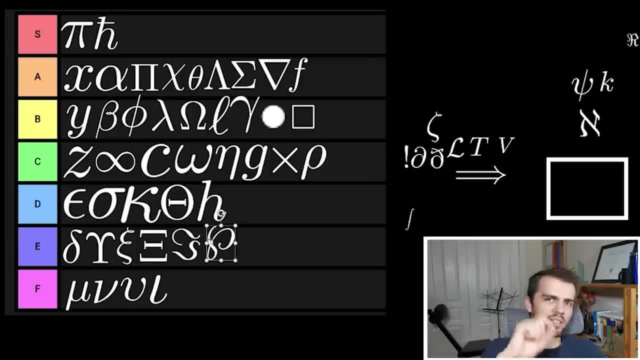 you know what? I need a new symbol and I'm going to just scribble. And then they come up with this and they scribble. I mean I'm telling you, whoever's making these, please stop Like it's just, it's too much. 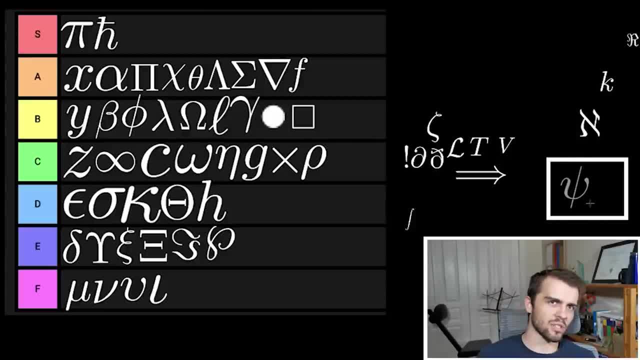 It hurts my head. Next we got Psi, And Psi is also holds a place in my heart: The wave function in quantum mechanics. What a beautiful symbol. You got that line striking down. get that nice little thing going through it. It looks like it's just pierced this part. 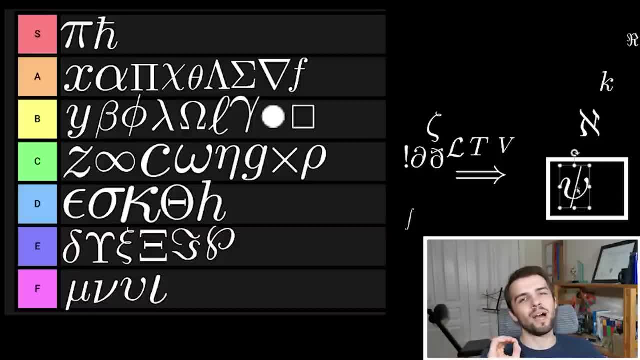 of it like a ribbon and it stabs right into the ground. My opinion: a lovely symbol, And this is an S? tier for its loveliness, The factorial. just an exclamation mark. Someone said this number is really big. We're going to have to mark it down with an exclamation. 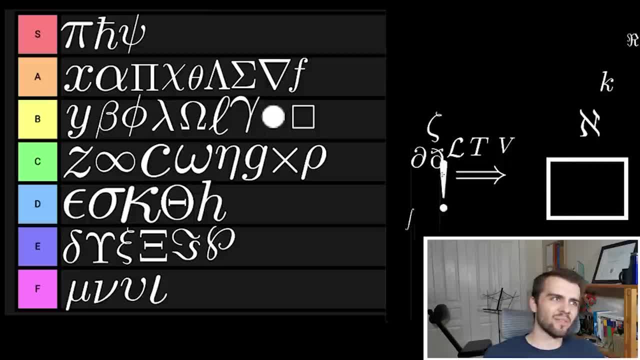 So you know, it's just, it's whatever. I think it's D tier. I don't even know what to say about it. Just is an exclamation mark. Partial derivatives, kind of cool. They're like you know what. 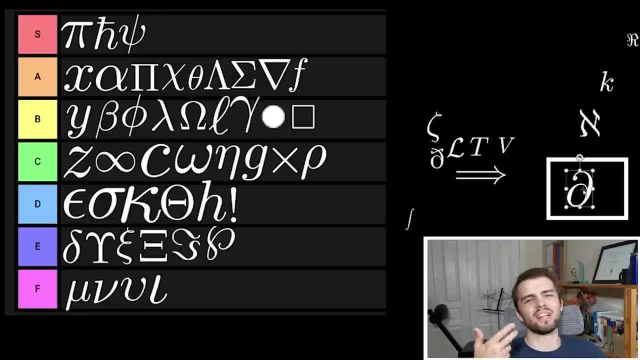 A derivative has a D. I want them to still know it's a derivative, but I don't want to mistake the two. I'm going to curl that top of the D and you get this symbol here And it kind of shows up in some dark places sometimes. 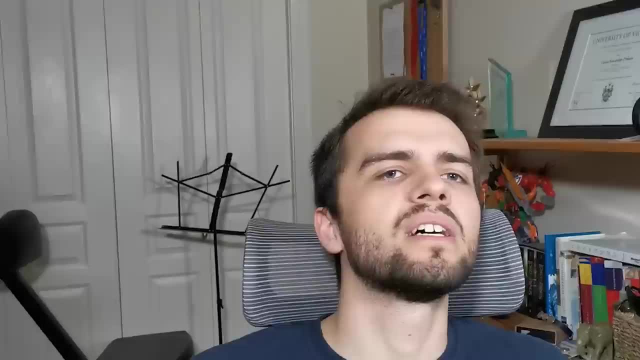 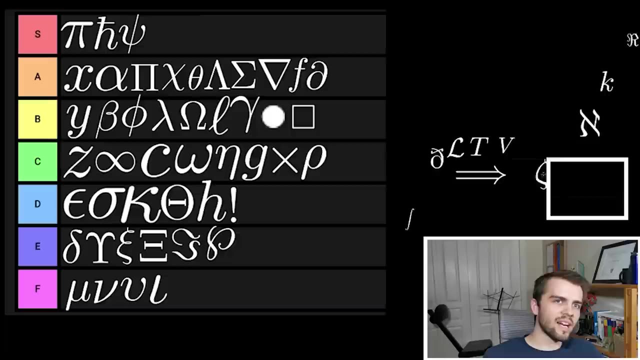 when you're solving something and you think, ah, partial derivative, what a pain. I think this is an A tier just for its functionality, especially, Again, another one of these squiggly symbols. If you use this on your paper, then you're pretentious. 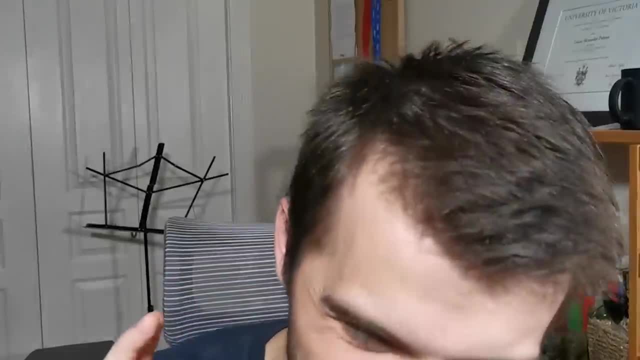 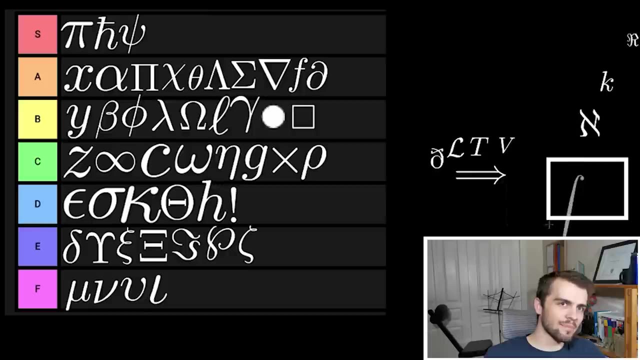 Just stop use another symbol. You don't need this. You really don't need this symbol. It's not required. This is an E tier symbol, The integral classic symbol. This was like one of the biggest advancements in math, obviously integrating. 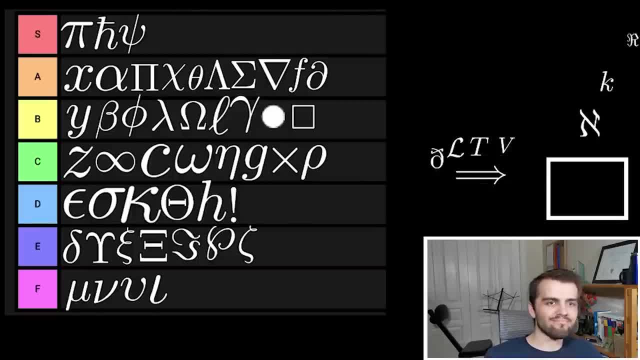 What a crazy thing. It's not. well. I'm sort of going to put it in between the A and the S tier, because it's too big for me to do anything. So it's sort of a mix there. I'll do that. 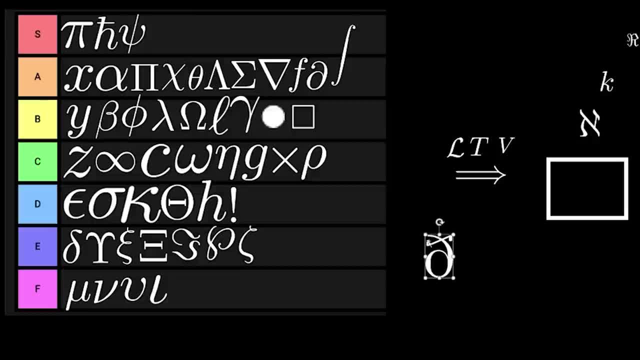 Actually got this symbol here. It's kind of like a partial derivative, but they're like: okay, now there's all this other stuff that we're going to do with the partial derivative. I remember dealing with this sometimes and it was really kind of. 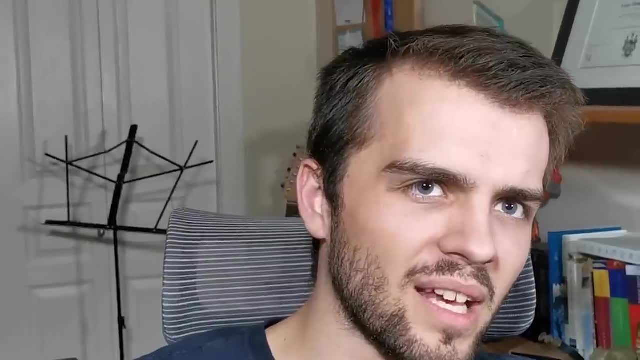 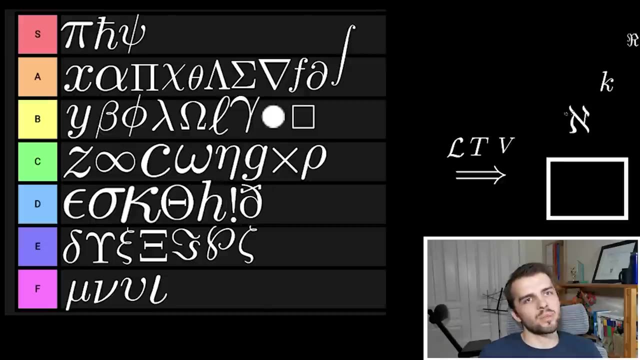 it was just not a good time. I remember not really even liking it, So ingenuity to the guy who came up with it. This is about a D tier symbol. Next we got the symbol Aleph. It looks like an N. that was like I'm the king of all Ns. 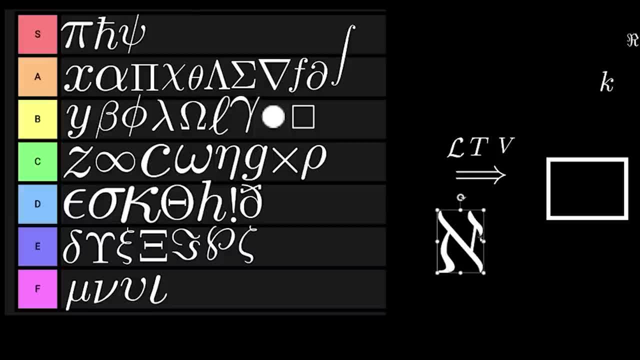 You know, it's got its foot down here with its leg And then it's got like a A And then it's got an X here. It's just, it's very fancy of a symbol. It shows up in Aleph, not the classic math symbol. 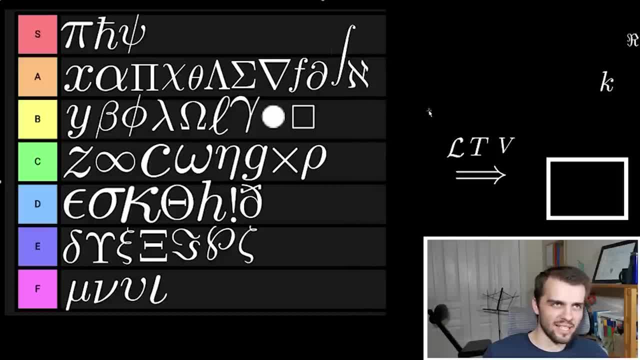 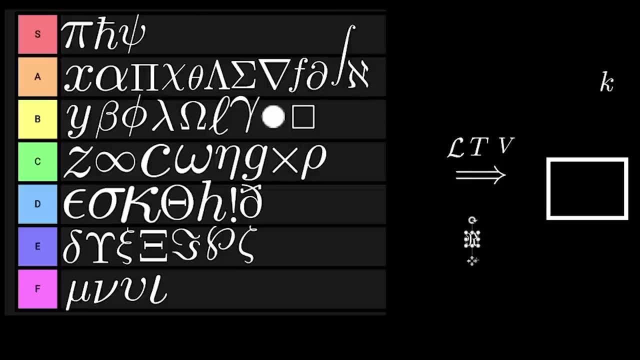 I think this is an A tier just because it is pleasing to look at, but it also is one of those painful looking symbols Like I would hurt myself if I was nearby it R. this is like one of these classic things, Like if you were to read an old like Shrek book. 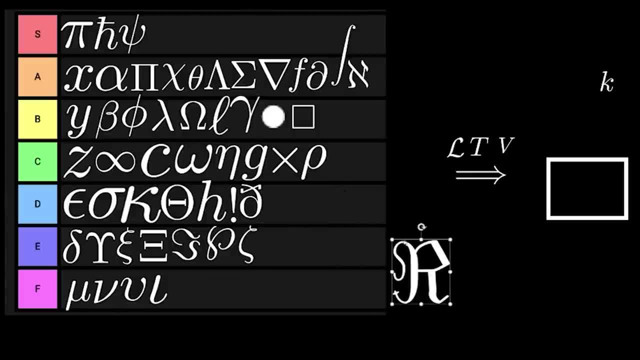 that Shrek was reading at the beginning and it's a fairy tale and it's just like I'm gonna read this book for knowledge. It starts with this big R, very fancy looking symbol. They even put this little tail here. There's a lot that went into the crafting of this symbol. 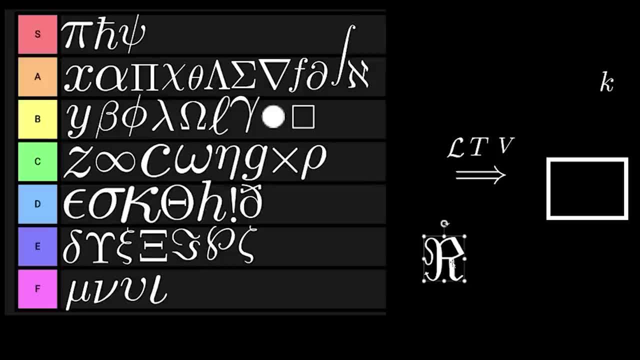 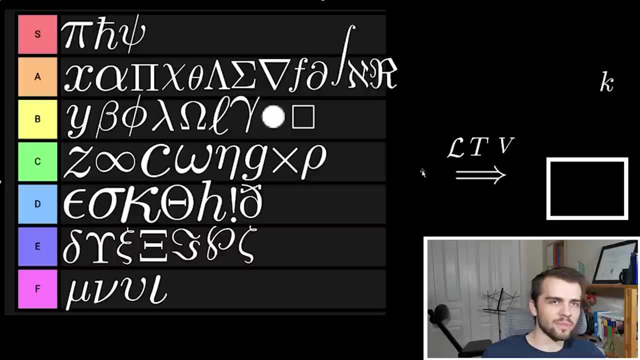 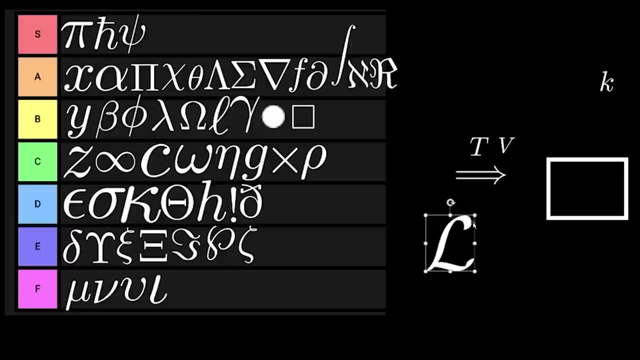 This represents usually the real component of a number. It looks nice. I'm gonna probably put it A tier. It's just a nice looking symbol. The L for Lagrangian. it's kind of nice. I don't know. It's got kind of a flow to it. 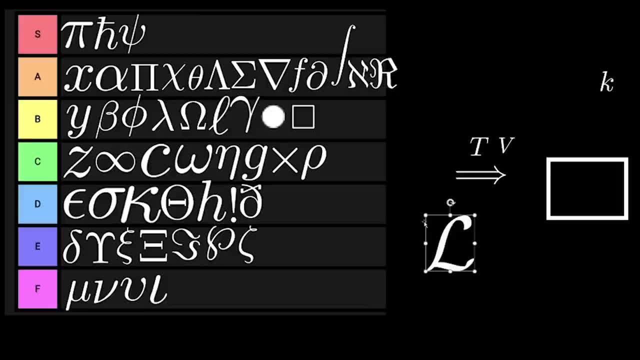 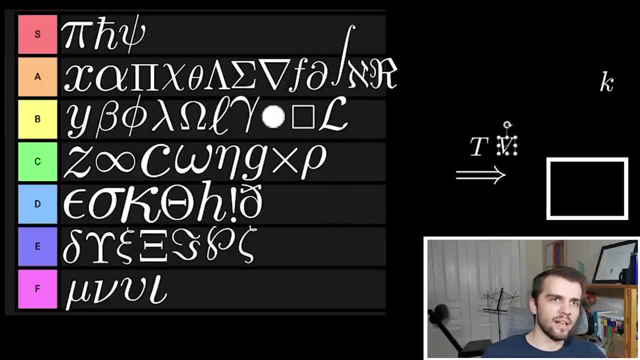 It's nice to write it with a loop when you're doing it on paper, but apparently it doesn't have that. here. I'm gonna put this B tier for being just a nice symbol. Now, the problem with V is that it's got potential. 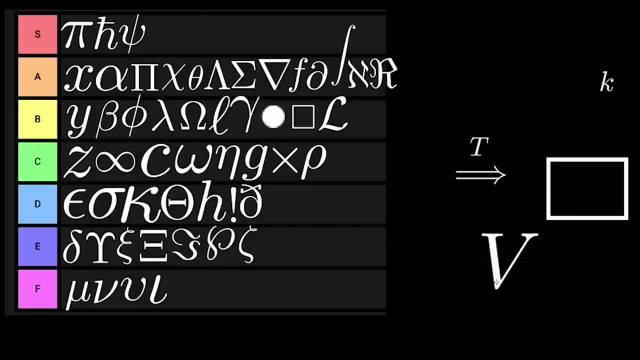 literally. but you know, I don't know why this is a lot thinner than this. Maybe there's some aesthetic thing that we like about that. I'm gonna probably put this B tier. I'm gonna probably put V and a C tier, along with capital T as well. 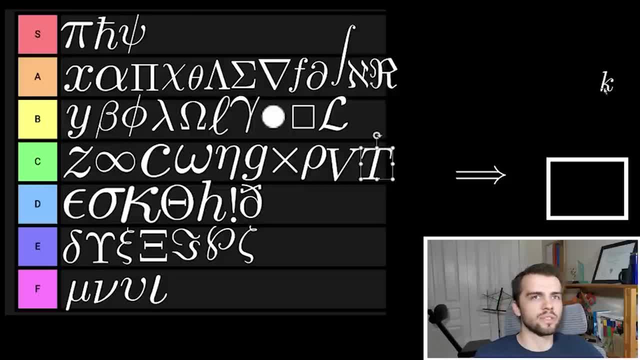 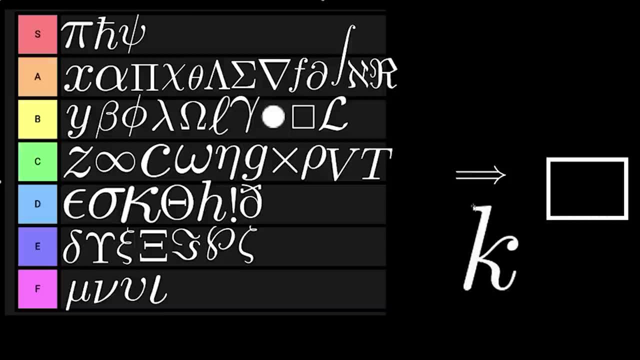 They're just overall decent, but nothing special to them. Finally, we've got Boltzmann Constant little K. Now this K's got a lot going on here. I don't really know. It's got this jutting out up top. 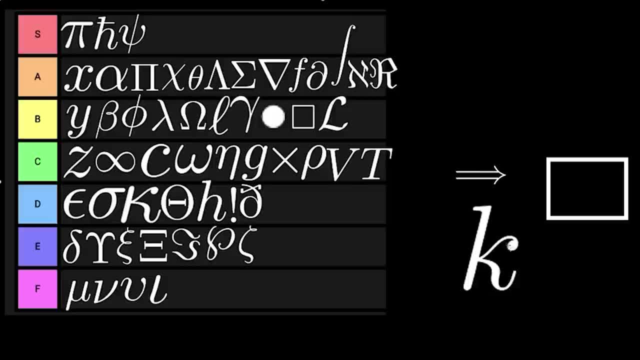 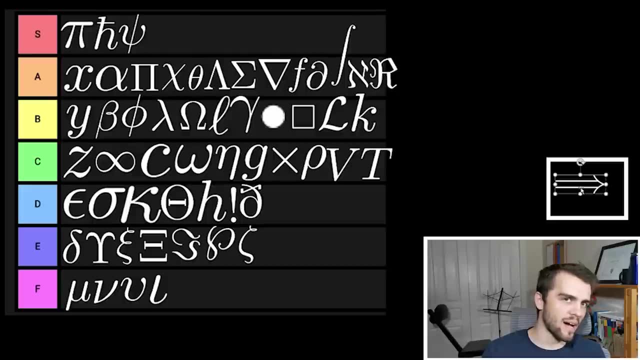 You got this kind of a hook here. You got this like it's unraveling something like a plant- almost Very interesting design choice. This is clearly going to be a B tier. Finally, the symbol implies- and now this is interesting- used for proofs and math. 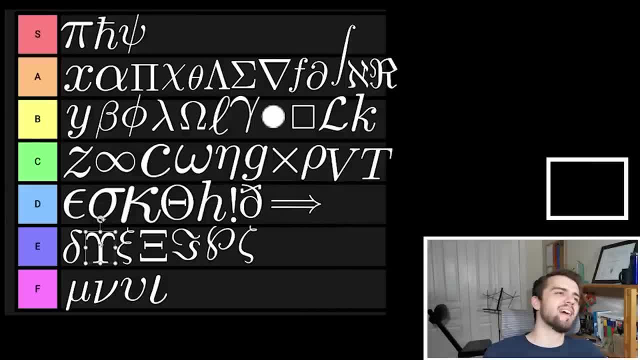 Nothing special about it. I'm gonna put this D tier. I mean, I think I was maybe unfair to this. I kind of like this and this is sort of the mystery one and this I think I'm gonna make it really large. 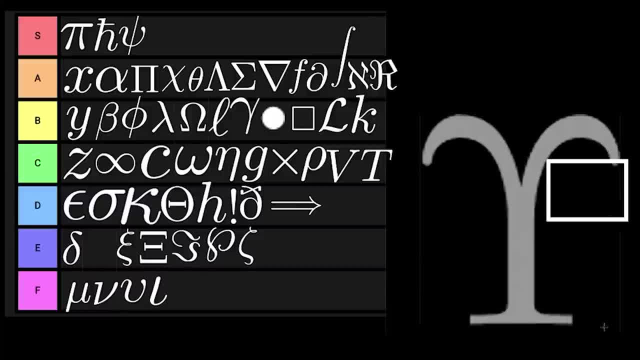 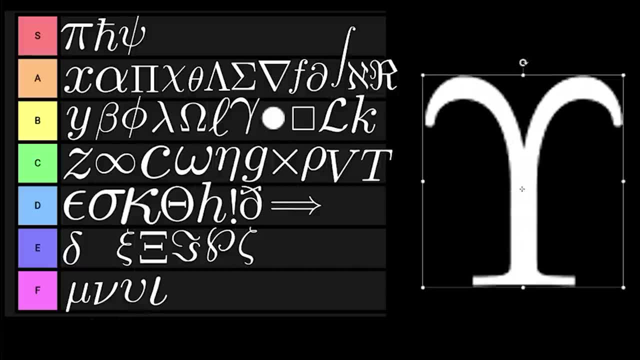 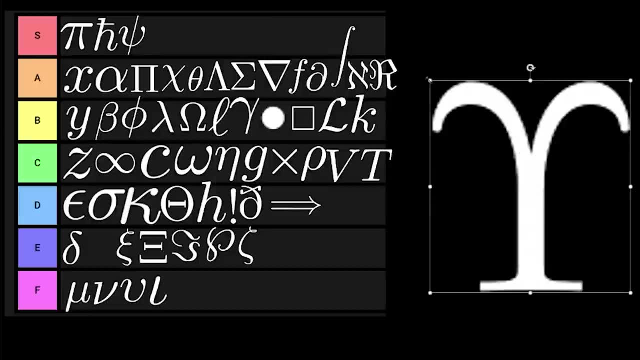 and just put it outside the tier list, because I think it's worth remembering that this exists. Remember it, So this belongs here in the advertisement symbol. I challenge everybody to use this symbol in a paper for now and if, for some reason, this video goes viral. 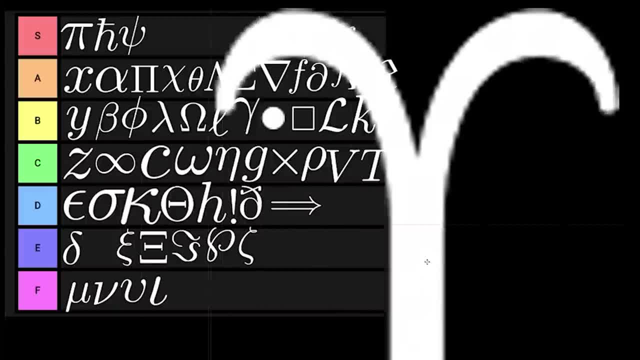 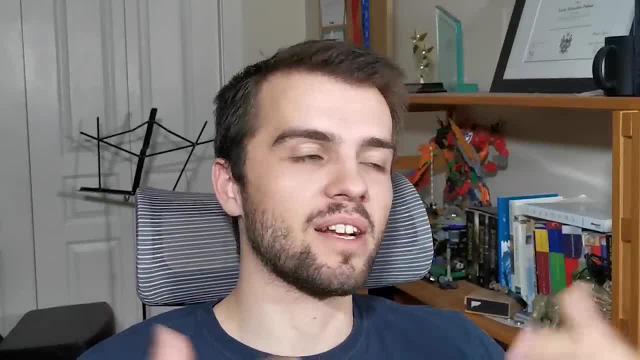 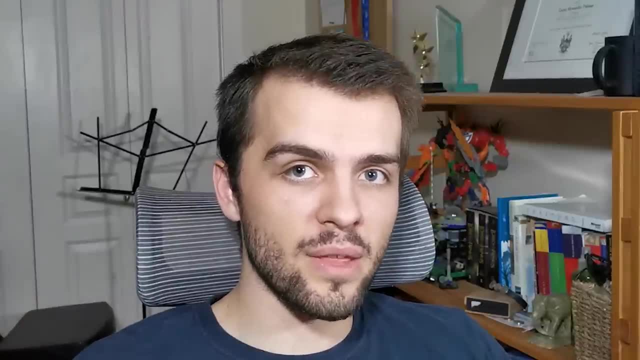 I hope this symbol you use. I hope you enjoyed this video. Be sure to like and subscribe for Python tutorials and other interesting topics that I just randomly come up with. Join the Discord server as well if you want to talk with other people in math or physics or anything. 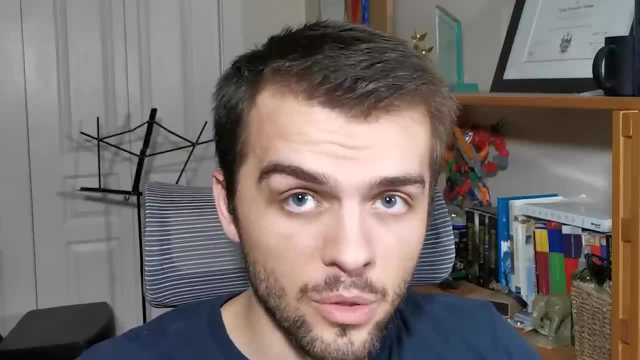 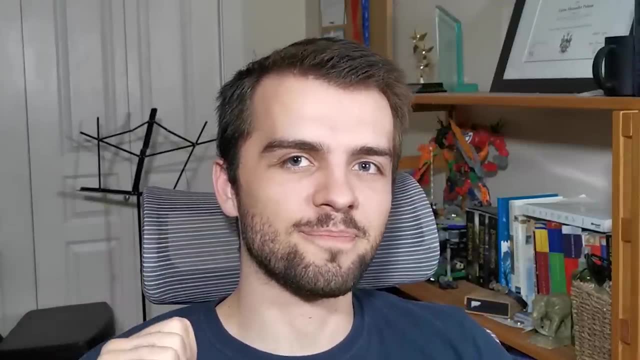 and you want to engage. There's been people talking about the various projects that they're working on, for example, and it's a very common thing. It's a very kind community of people, so join that as well, and I'll see you next time.